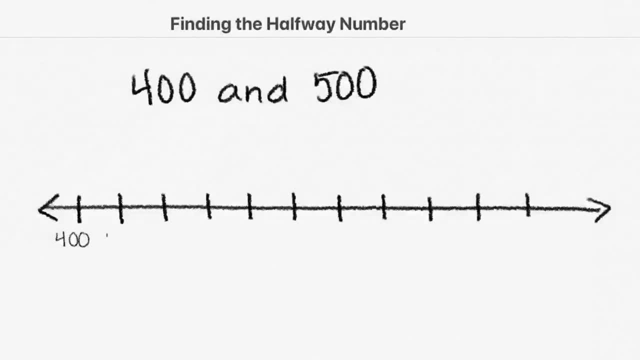 numbers 400,, 410,, 420,, 430,, 440,, 450,, 460,, 470,, 480,, 490, and 500.. Now it's important to notice that if we would have gone by ones or by fives, it wouldn't have fit using just 10 tick marks. 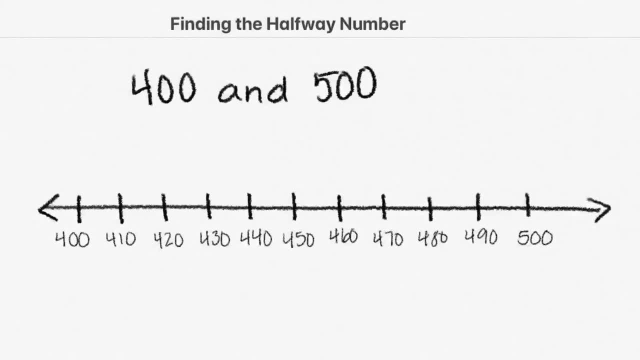 So that's why we went by tens. Now we will jump inward from both ends: One, two, two, three, three, four, four, five, five, And that's exactly where they meet halfway at 450.. So halfway between 400 and 500 is 450.. Let's find halfway between 100 and 200. 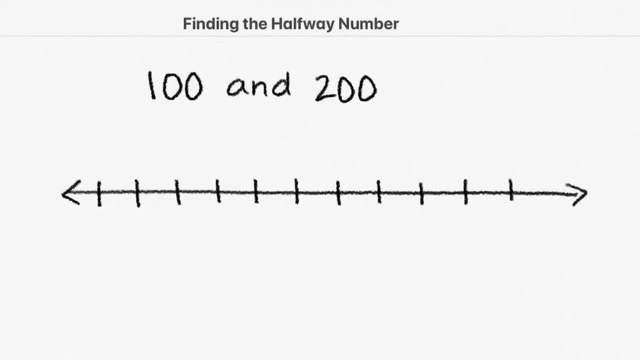 And remember, we only have 10 tick marks, so we're going to have to skip every 10 tick marks. So we're going to have to skip every 10 tick marks. So we're going to have to skip every 10 tick marks in order to fit 100 all the way to 200. 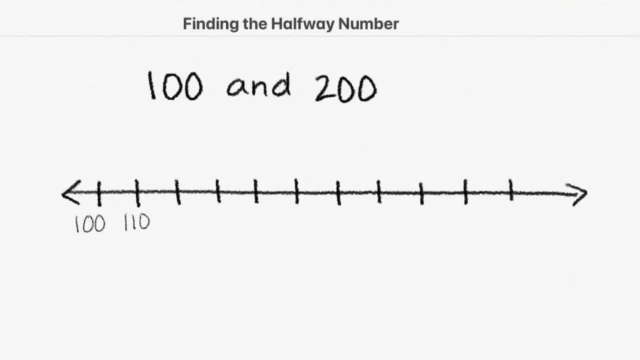 Let's label our number line 100,, 110,, 120,, 130,, 140,, 150,, 160,, 170,, 180,, 190, and 200.. Now we have to jump inward from both ends: One, one, two, two, three, three, four. 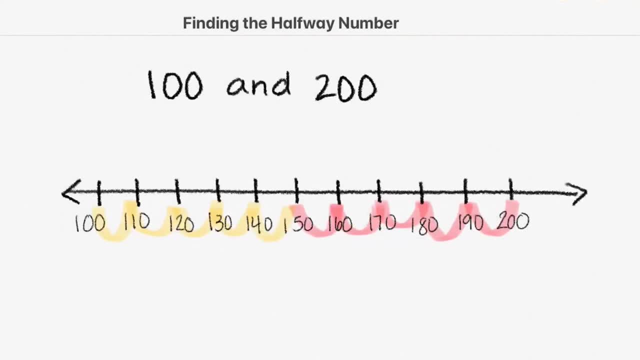 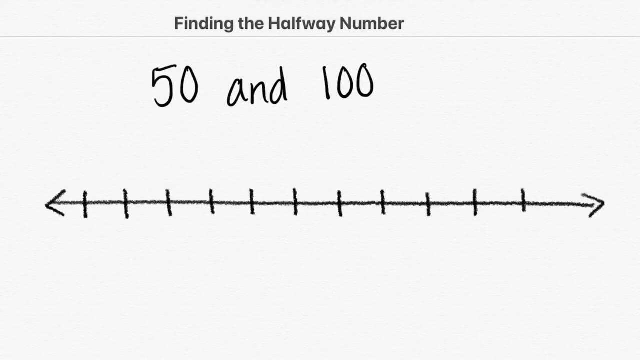 four, five, five, And that's where they meet halfway at 150.. Halfway between 100 and 200 is 150. Now we're going to find halfway between 50 and 100. If we jump by ones, there won't be enough. 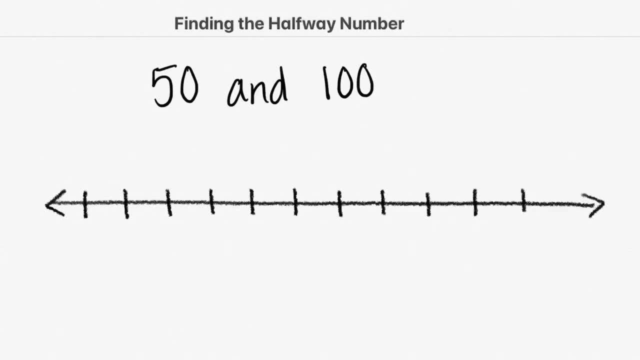 space. If we jump by tens we would have too much space left over, So we're going to have to jump every five numbers: 50,, 55,, 60,, 65, 70,, 75, 80,, 85,, 90,, 95, 100.. Let's begin jumping inward from both ends: One, one, two, two. 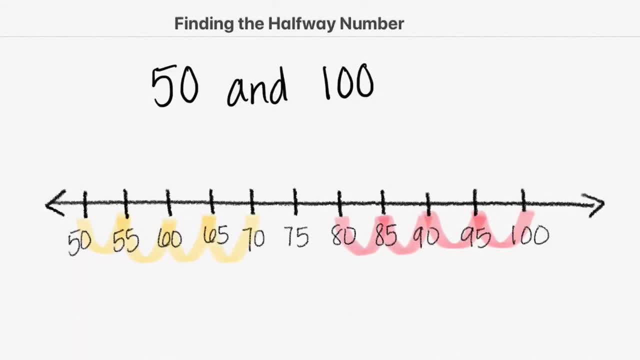 three, three, four, four, five, five, And that's where they meet halfway at 75.. Halfway between 50 and 100 is 75.. Let's go.